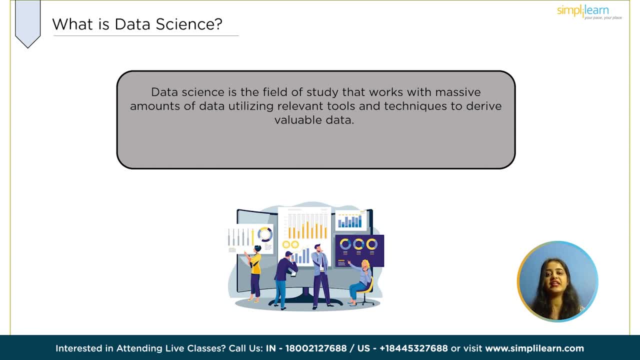 work of a data scientist involves collecting, analyzing and interpreting this data to help businesses achieve their goals. The role of a data scientist is to extract raw data and convert it into meaningful information. If we must define data scientist, they are the people who make. 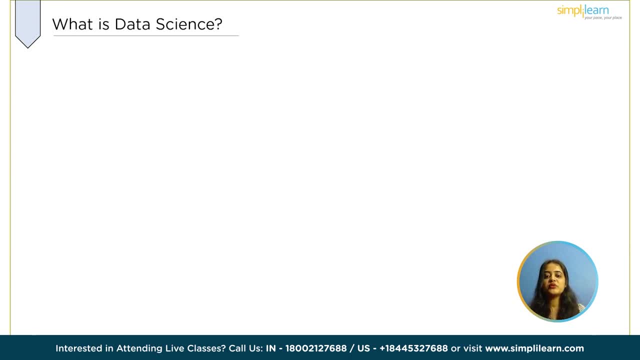 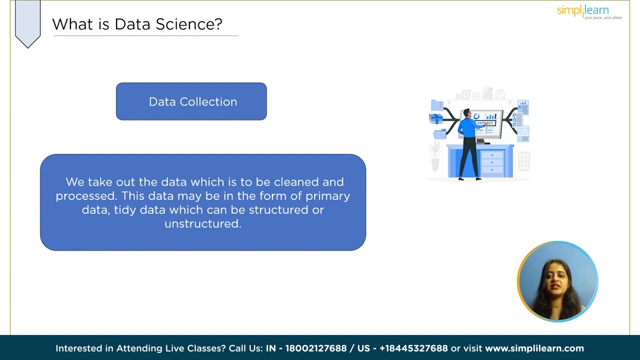 value out of invaluable data or raw data. Coming to stages of data science, it has mainly five stages. First is data collection, or acquisition. In this stage, we basically take out the data which is to be cleaned and processed. This data may be in the form of primary data, tidy data which can be structured, or unstructured form. 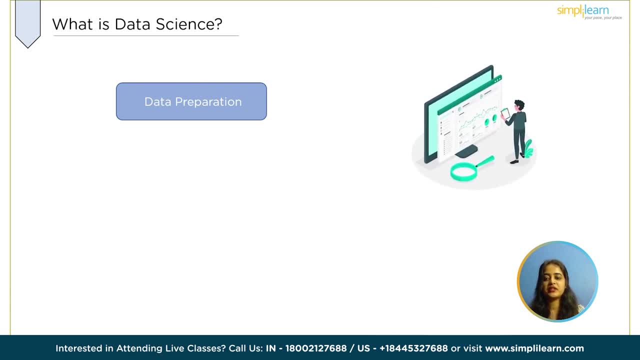 Next is data preparation. The data collected during data collection is processed or treated in the states. Raw data cannot be processed directly. Eliminating inconsistency in data happens in this stage, For example, removing blank spaces, special symbols or anything that is irrelevant in the column, before it gets handled for further processing. 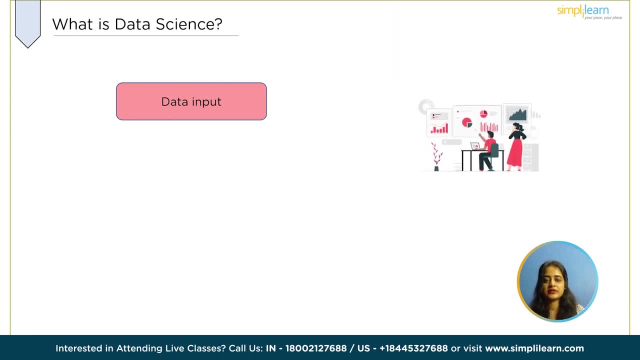 Next is data input. This stage is defined as the task of coding and converting the prepared data into computer readable data so that it can be processed using different software applications. Coming to data processing stage, This is the stage where we use artificial intelligence algorithms. 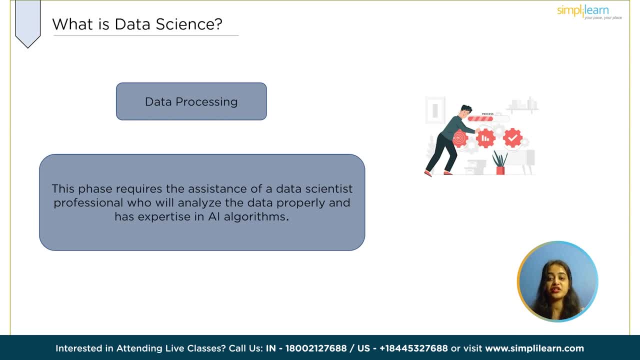 This phase requires the assistance of a data scientist professional who will analyze the data properly and has expertise in AI algorithms. And the last stage is data interpretation. In this phase, we have got data which is totally cleansed and it is to be used by the user. 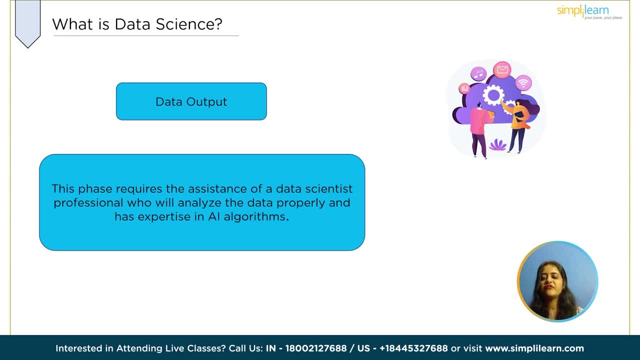 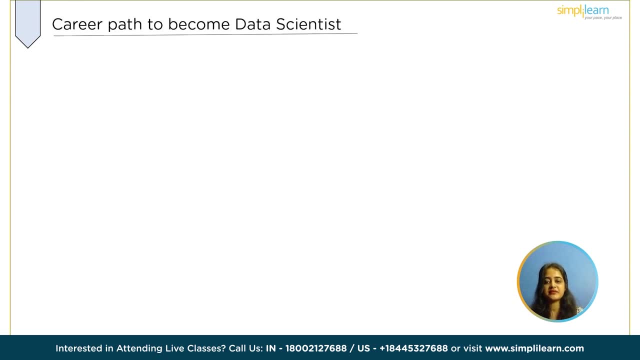 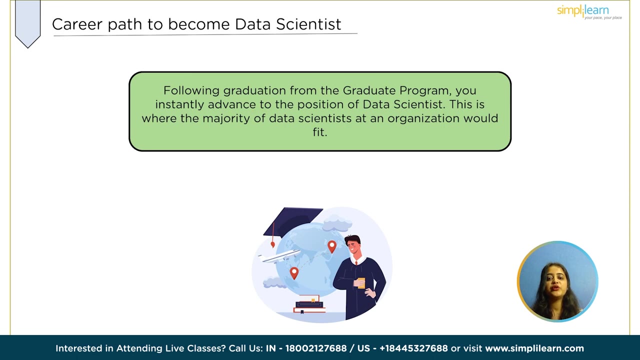 It can be audio, video or graphical data. We have understood the fundamentals of data. Now it's time to learn qualification to become data scientist. Basic bachelor degree is enough for a data scientist. As a data scientist, you need to know about fundamentals of mathematics, statistics. 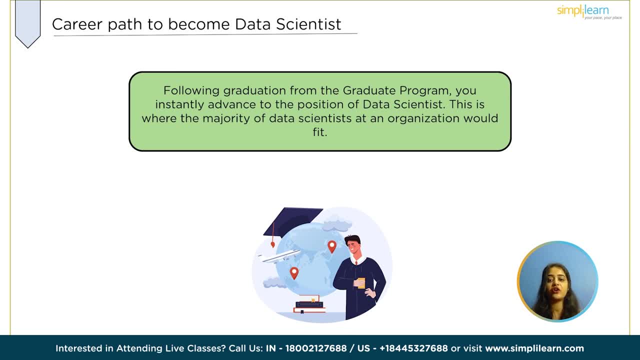 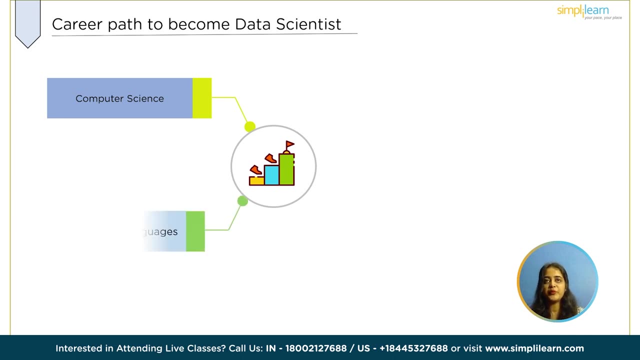 After that, learn machine learning algorithms as well as AI algorithms. Along with that, please go through important programming languages for data science like Python and R. Practice any of these languages. So we need computer science, programming languages, mathematics and statistics and finally, machine learning algorithms, to master data science. 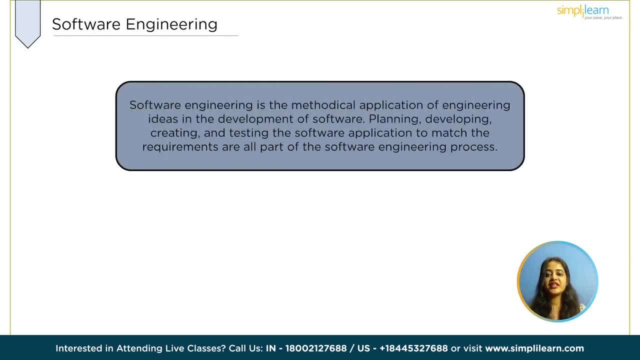 Now, what is software engineering? Software engineering is the methodical application of engineering ideas in the development of software. Planning, developing, creating and testing the software application to match the requirements are all part of software engineering process. It is one of the most popular careers, for a reason. 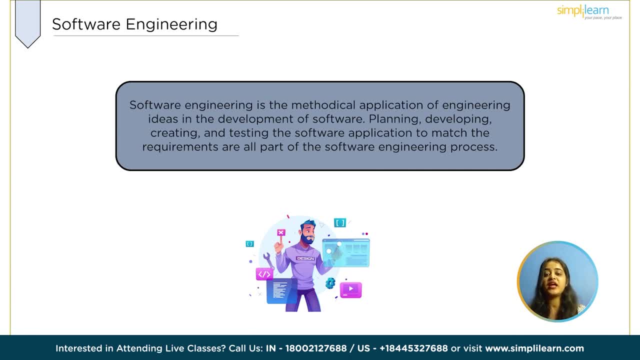 Software engineering is a comprehensive study of engineering applied to the design, development and maintenance of software. Software engineers use a variety of programming languages and tools to design, test and deploy software solutions. They are in charge of creating and maintaining software applications. Software engineers must have the ability to diagnose problems and solve complicated challenges, in addition to producing code. 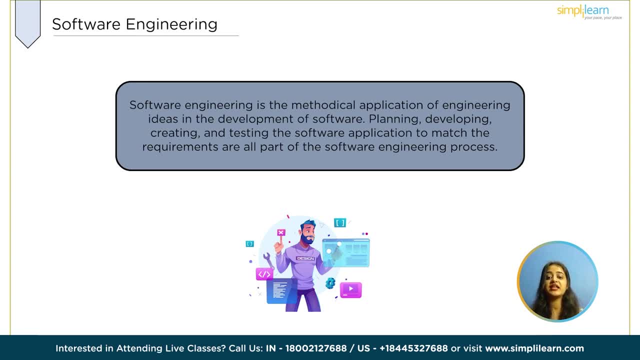 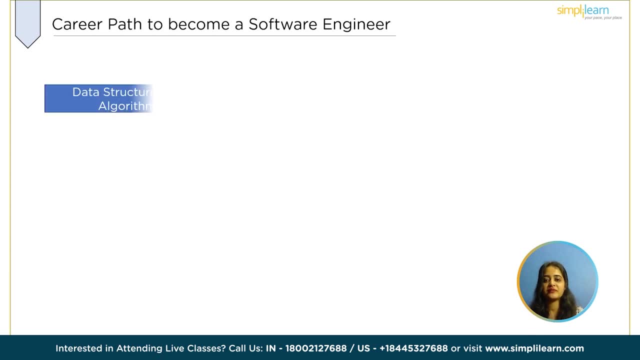 Software engineers must have the ability to diagnose problems and solve complicated challenges, in addition to producing code. The need for knowledgeable software engineers is increasing, along with the need for fresh and good software solutions. Now qualifications needed for a software engineer? Firstly, as a software engineers, you will work on design, development and testing of software. 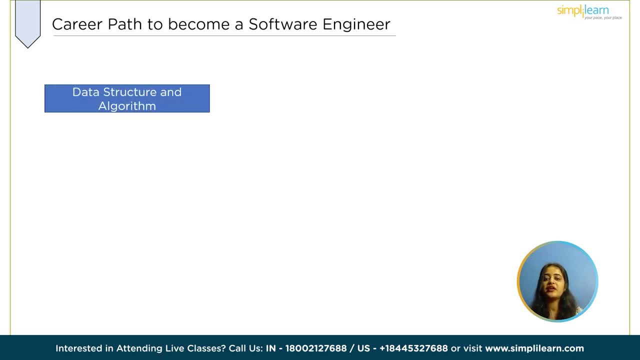 For that, firstly, we need to learn about data structure and algorithms. After that, start learning coding languages like C, C++ and Java. After that, you need a biennial degree in software and computer science. You will also need to learn the necessary arb dào of coding languages. 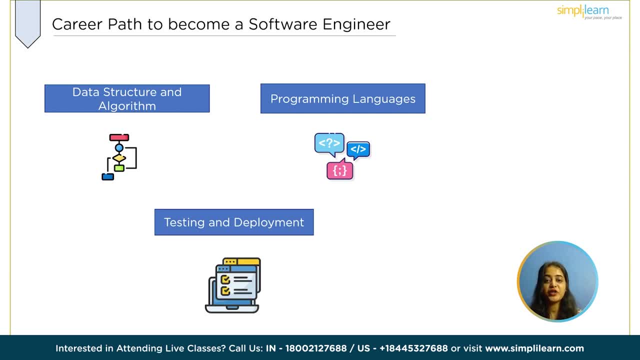 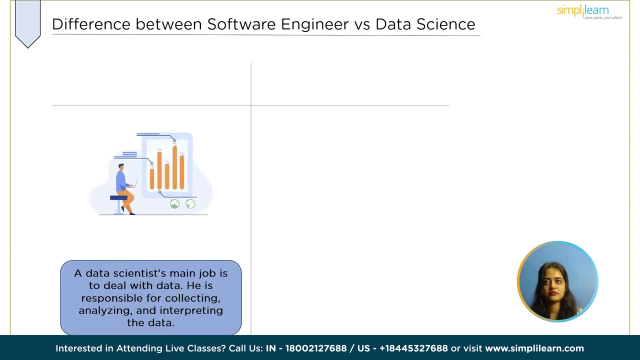 also need to learn about testing tools. if you want to become a QA, Don't be scared. any one of the programming languages can be considered. No need to learn C, C++ or Java. Coming to Differences between Data Scientist and Software Engineer Role played by a Data Scientist: A data scientist's main job is to deal with 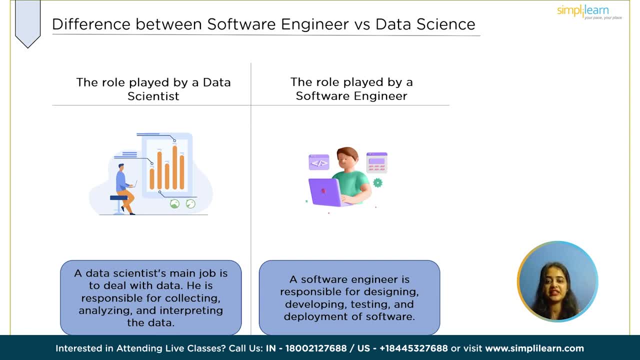 data. He is responsible for collecting, analyzing and interpreting data Here. as a data scientist, you work with a team to develop data strategy. It requires a lot of algorithms and tools. We will discuss the required tools later. Engineer. A software engineer is responsible for designing, developing, testing and deployment of software. 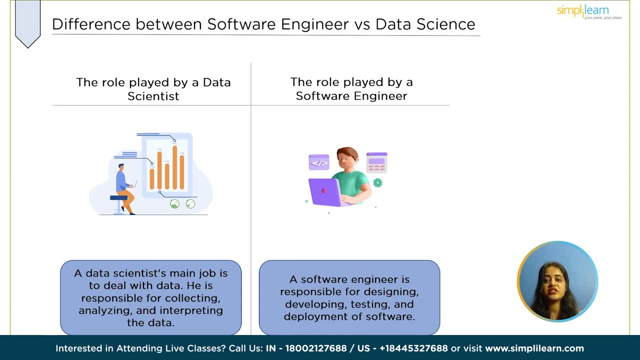 as we already discussed about this. As a software engineer in an organization, your role is to develop, test and deploy your software based on the requirement- information that you can very important in developing a software product. a software engineer is responsible for maintenance of the software. to now that we understood. 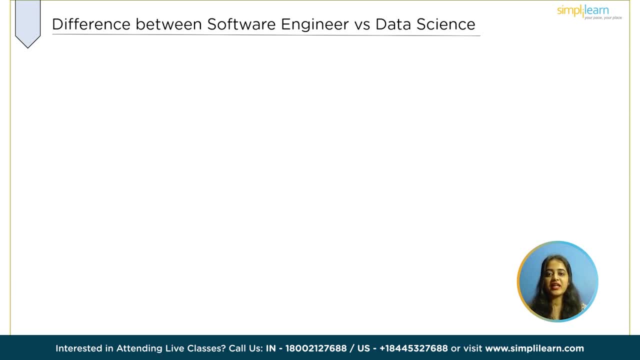 fundamentals of data science and software engineering. it is the time to understand differences between both of them. coming to role played by a data scientist, a data scientist main job is to deal with data. he is responsible for collecting, analyzing and interpreting the data. here, as a data scientist, you. 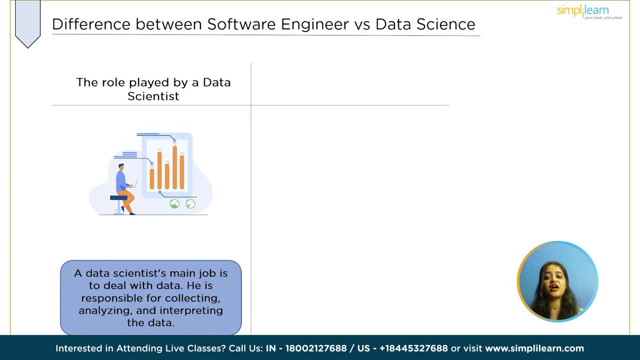 work with a team to develop data strategy. it requires a lot of algorithms and tools. we will discuss about required tool later. coming to software engineering, a software engineer is responsible for designing, development, testing and deployment of software, as we discussed about it earlier. as a software engineer in an organization, your role is very important in developing a software. 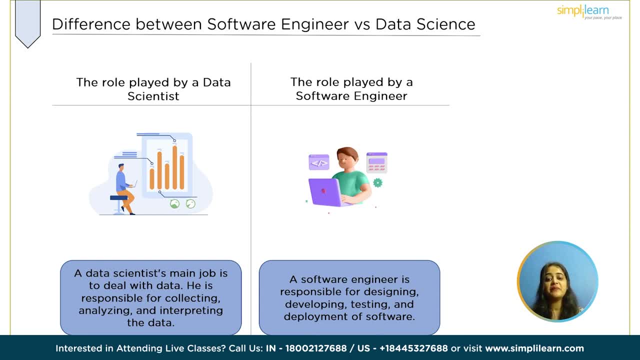 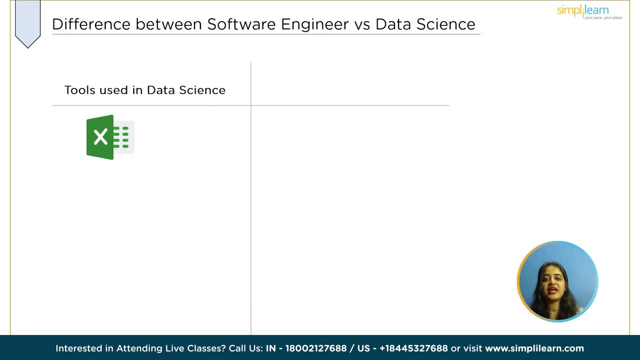 product. a software engineer is responsible for maintenance of the software to you. work with a team to develop data strategy. it requires a lot of algorithms and tools. we Next is tools used in data science. Data science adopts tools like Excel, Tableau, ggplot2, MATLAB, Apache, Spark, etc. 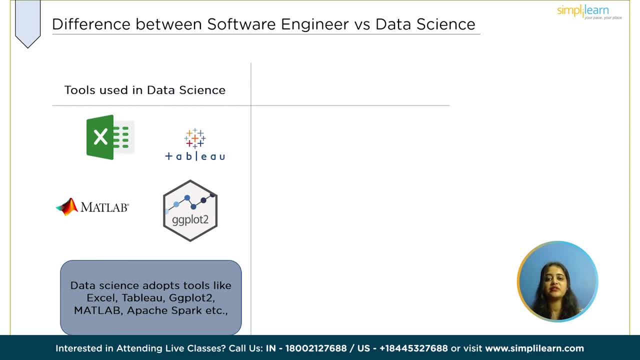 Among all these, Tableau is simple and easy to learn. For larger data sets, you may include Hadoop, MapReduce, etc. Coming to tools used in software engineering, as a software engineer, you can go with GitHub. Opting IDE is based on the programming language you choose to work. 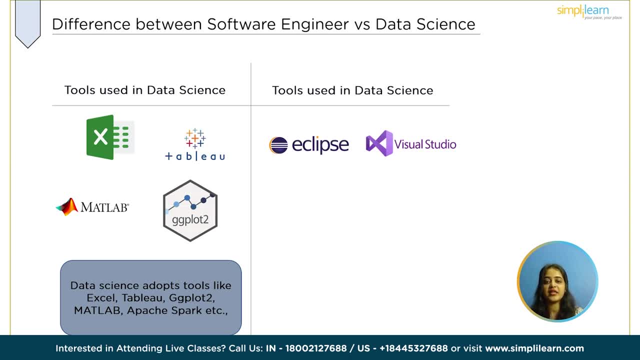 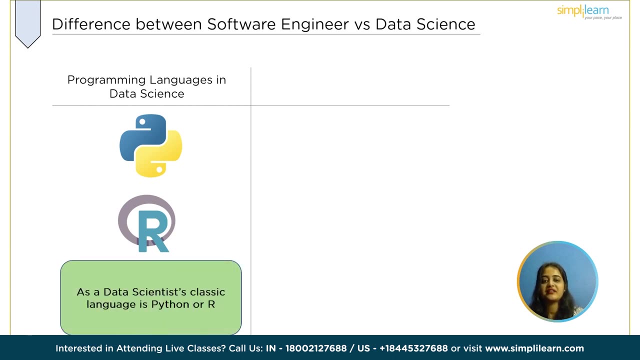 For instance, if you use Java, then it's better to choose Eclipse, NetBeans, etc. If you are choosing C++, then Visual Studio Code and NetBeans etc are preferable. Coming to the programming language as a data scientist, classic languages used are Python or R. 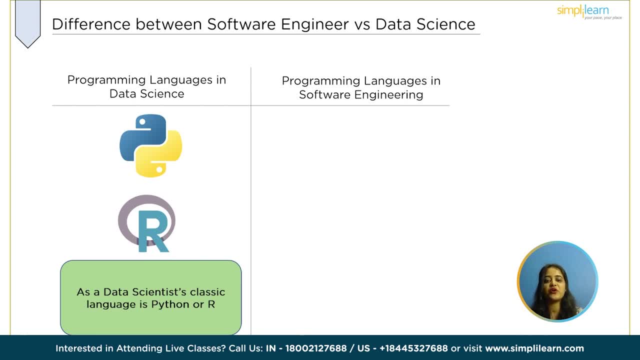 Best preferred coding language for a software developer depends on the application. Commonly used ones are C, C++, Java, Python, etc. For web development, P Use HTML, CSS, Bootstrap and JavaScript, And for database management we use MySQL, PostgreSQL, to store the data. 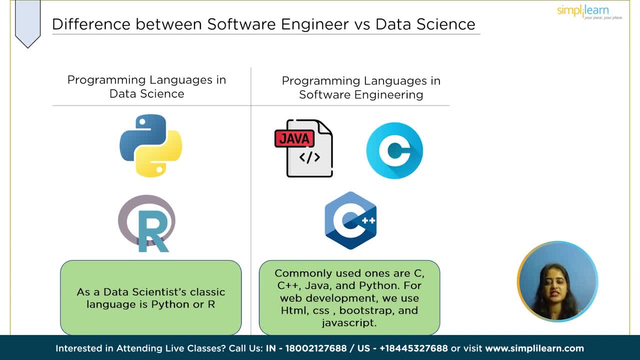 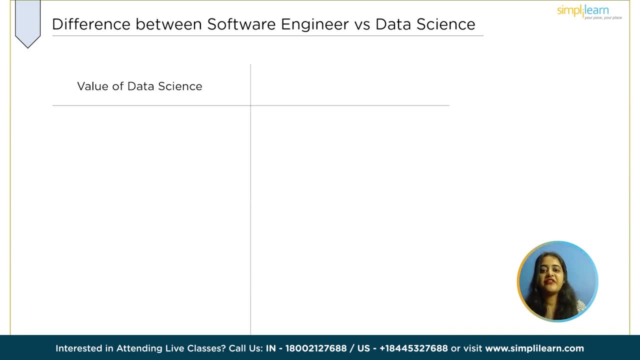 Finally, in testing we have manual and automation testing, But commonly used testing is automation testing. Now we will understand why we need a data scientist. Every company deals with lots and lots of data. Extraction of valuable data is required for the growth of any organization. 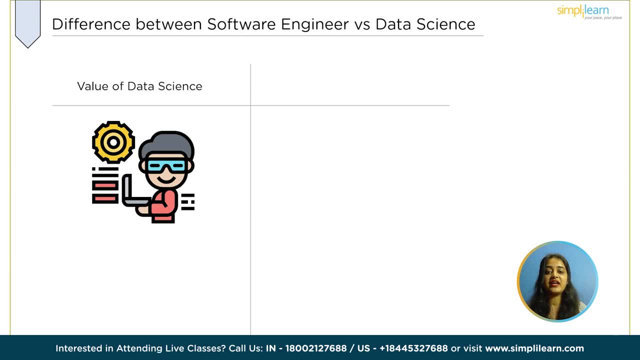 Therefore, the demand of a data scientist is very high Compared to any other position in the market. Around 1 million jobs are currently available in the world for a data scientist. Such is the demand of a data scientist. So software engineers are responsible for large projects with speed and less time. 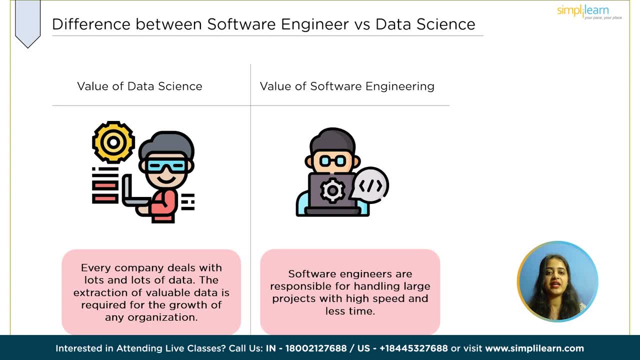 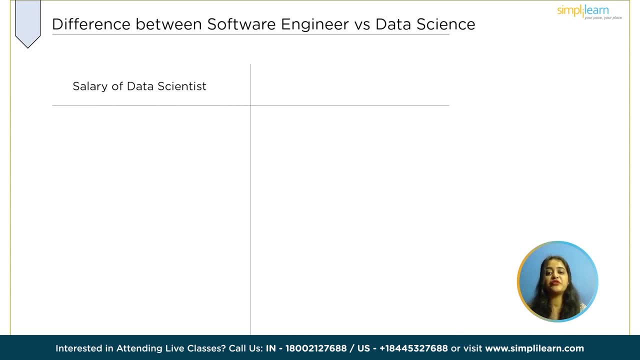 So the role of a software engineer in a company cannot be negligible at all. Moving on to salary of a data scientist: Reward is the result of a good work. Now we shall discuss salaries. What are the salaries that a data scientist will get? 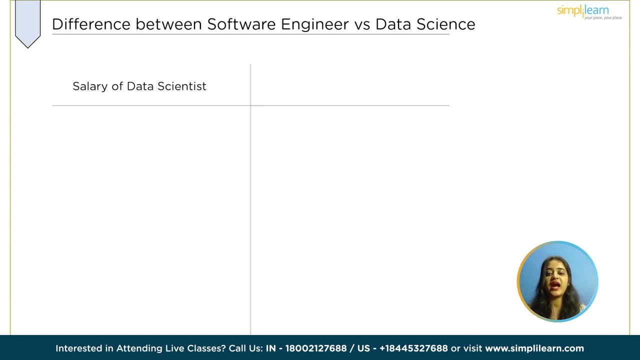 It should come as no surprise that data scientist may add significantly to a business. At the beginner level, a Data Scientist makes $95,000 US Dollars annually. The typical annual compensation for a mid-level data scientist is between $130,000 and $195,000. 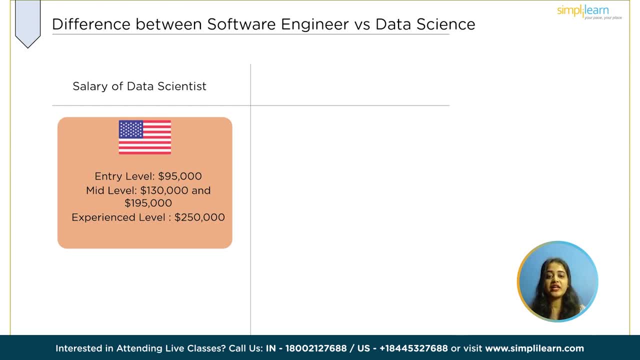 A seasoned data scientist typically earns between $165,000 up to $250,000. million dollars per year, depending on the level of experience. salary of a software engineer in US entry level is sixty three thousand dollars, but mid level is increasing to eighty six thousand dollars to one hundred thousand. 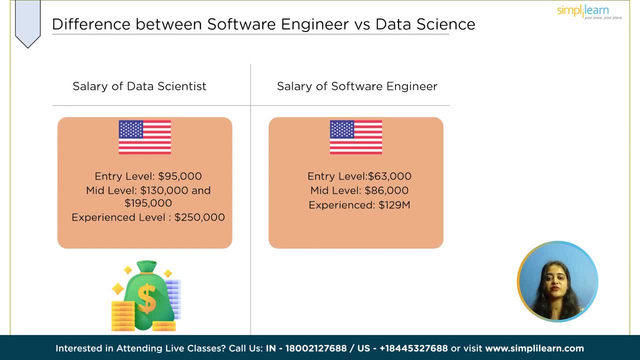 dollars experienced, one can get one hundred thirty thousand dollars. it can vary from company to company, but we have discussed this average salary in this video. coming to salary offered for a data scientist in India, in India, at the beginner level, a data scientist makes rupees nine lakh forty thousand on. 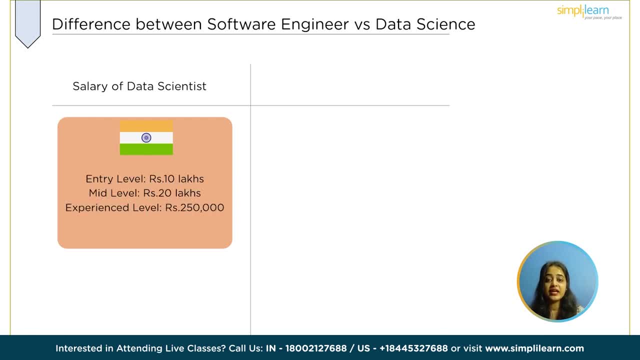 average per year. at mid level, a data scientist will get rupees 20 lakhs per annum to and if you are at advanced level, you will get paid an average salary of rupees 25 lakhs annual. coming to software engineer at beginner level, a software engineer will get average salary. 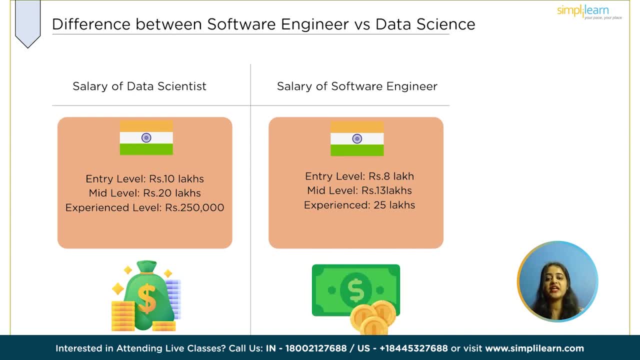 at the beginner level, a software engineer will get average salary at the 8 lakhs per year. A mid-level, experienced software engineer will be rewarded with the salary as high as 15 lakhs per year. A senior software engineer will be rewarded with a salary of 30 lakhs per year. This is according to indeedcom.